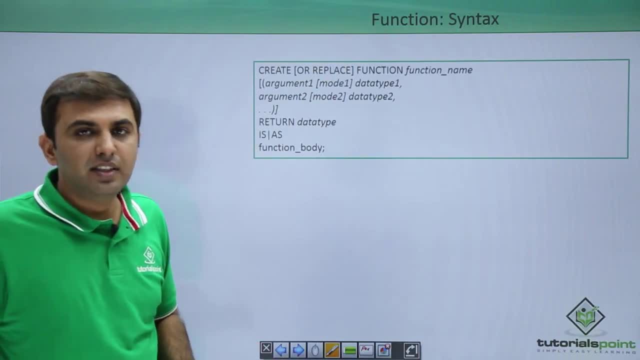 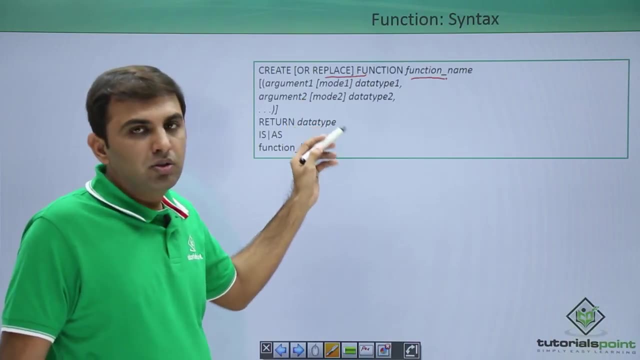 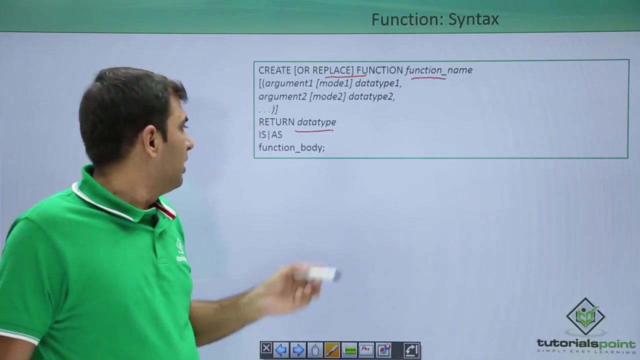 Next, functional syntax. So functional syntax is similar. So functional syntax is similar. So functional syntax is similar to the procedure: create or replace function function name arguments. here you can also define in out or in out, whatever, and return is the extra thing. return data type, because function always return some values, and here is as function body. 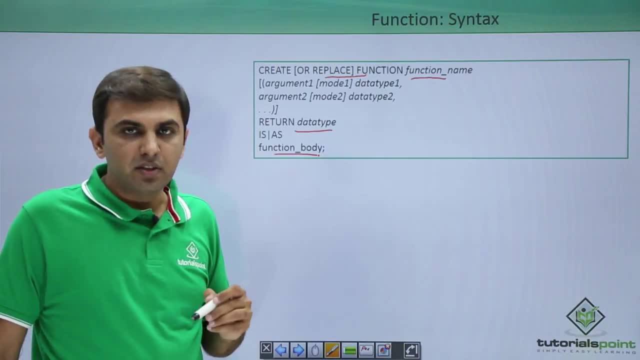 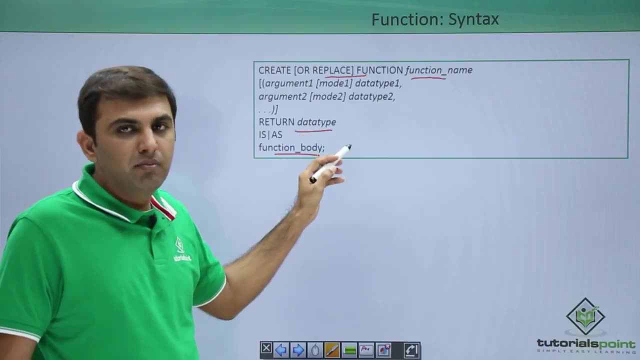 Fine, here you can just write down the begin section, exception section, end section. So this is the syntax for the function. The only difference is that it is returning the value, and here you have to write down the return data type, whether it is a number or worker. 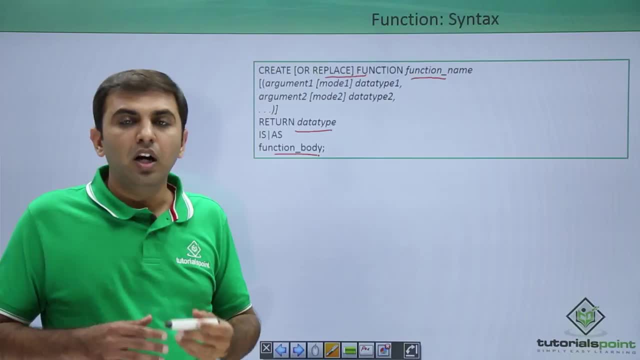 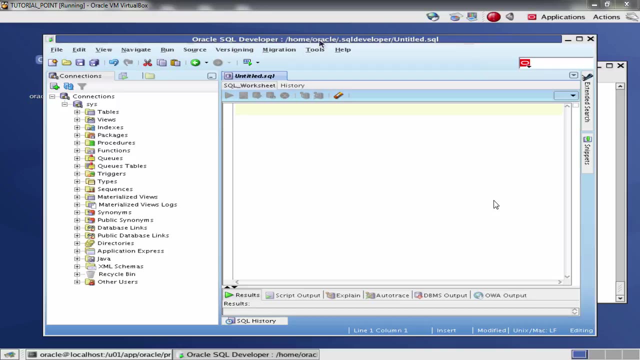 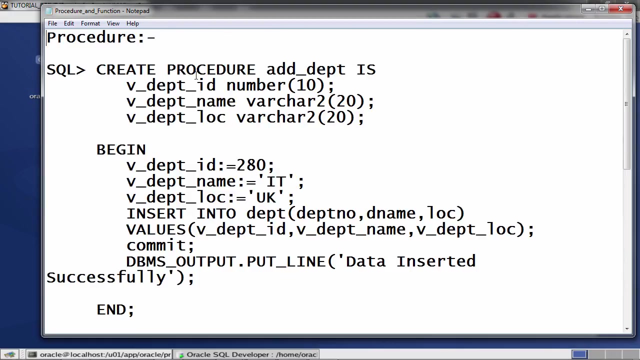 So let's see the practically how to create procedure, how to create function and how to execute procedure and function. Let's see how to create store procedure and function in oracle database. So first we are going to create store procedure. So we are creating the store procedure to add department in your dbt table. 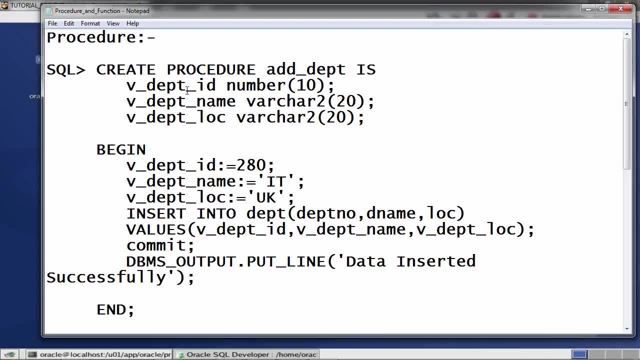 So we are declaring the three variables. So we are declaring the three variables inside the procedures: Create procedure. procedure name is add underscore dbt. These is the three department. sorry, three variables we are just defining, Fine, and here we are just assigning value to this: three variables. 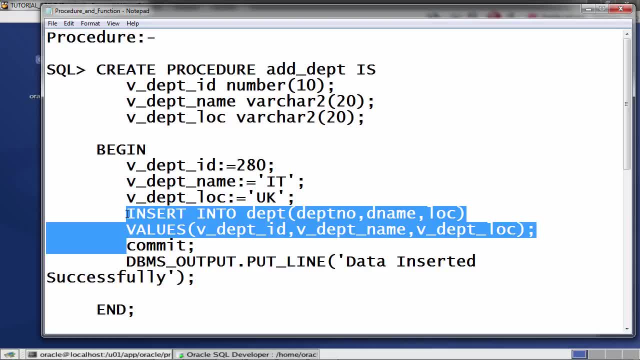 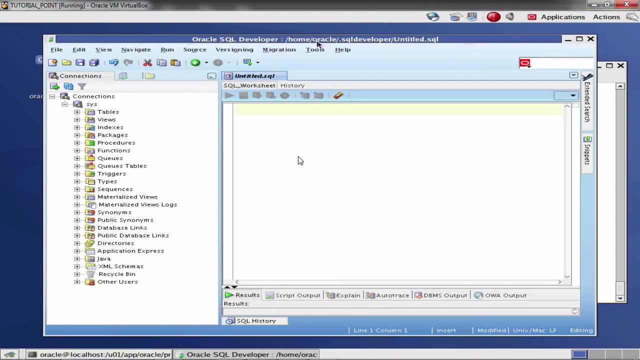 After that we are inserting the values into the table and committing and at the end we are just printing the output Data inserted successfully. So let's see practically Create procedure We are creating in SQL developer. Create procedure Procedure. name: add: dbt is v underscore department number. 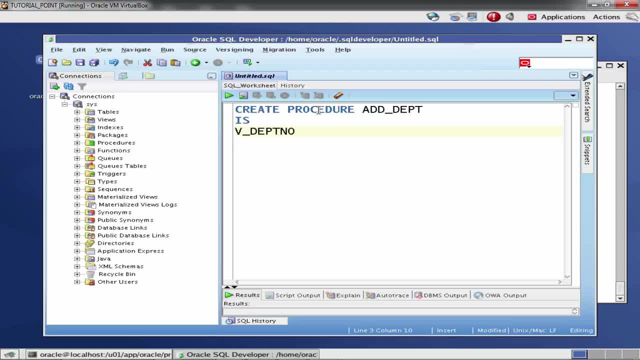 So v underscore. v means here we are just writing v underscore. whatever the name you want to give, you can give, But here we are just writing v underscore. But here we are just defining v underscore department number. That means variable underscore department number. very good number. 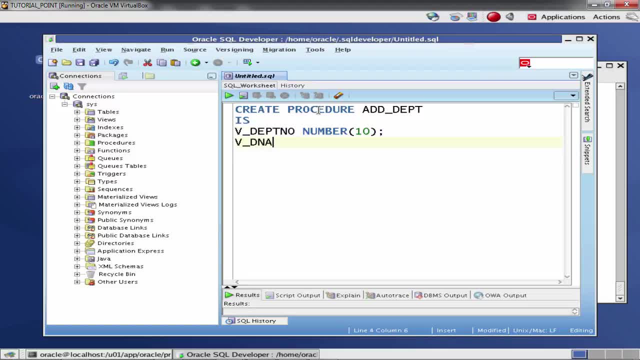 That is the number. Thank you, I hope it helped you. Bye, Bye, Bye. And here we are just defining the u underscore department number equal to. I am just defining the values to the variable and here I am just search department. let us see, that is location. 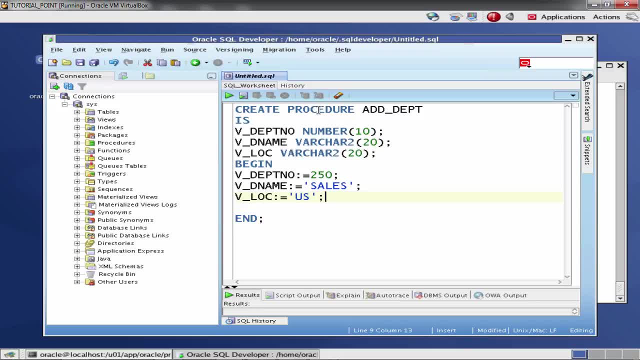 I am just giving to the. whatever the value you want to give, you can just give. So here I have just created three values. I have given three variables and assigning value to this. three variables insert into add dept values and values. I am just giving u underscore dept number, fine, and I am just 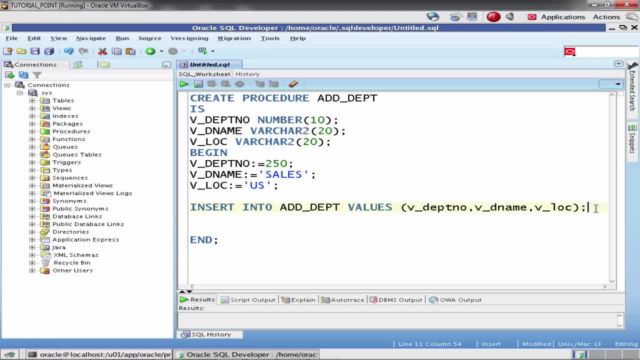 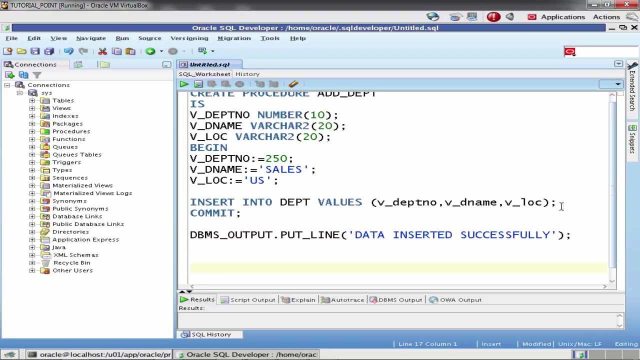 committing the data. Sorry, I need to just write down the dept. I am just printing the data inserted. fine, So here, initially, first of all, you need to just create this procedure. it is not like an anonymous block At this moment. you need to just create the procedure and this procedure is initially. 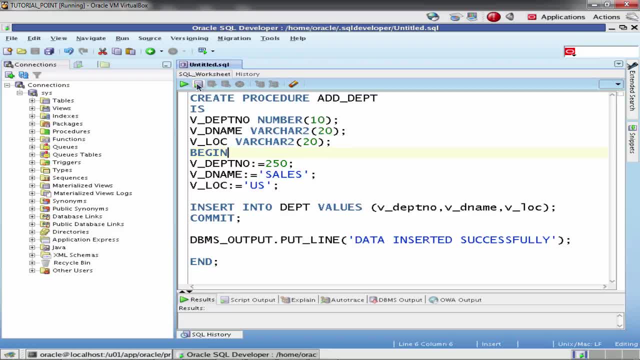 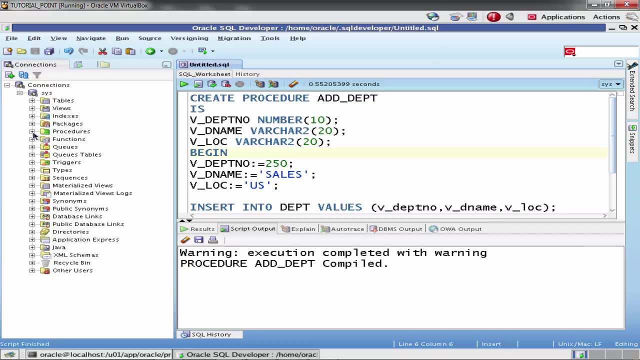 it is compiling. so, in case, if you have any syntax error, so that syntax error is going to be displayed over here whenever you are compiling. So let us see any syntax error is there or not. So some warnings are there. so let us see. just go to the procedure on the left hand. 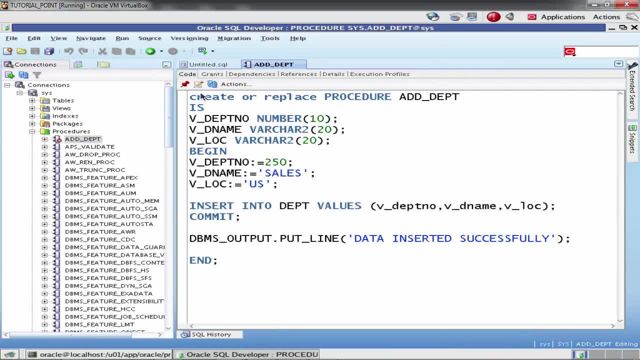 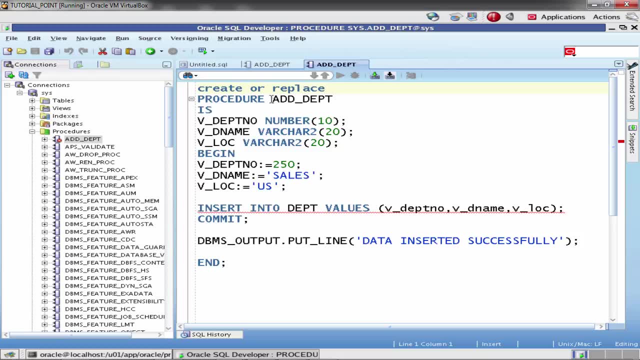 side. just add department. What is the So here insert into dept. so this dept not available. so scott dot dept. need to write down dept number v underscore d name and v underscore loc. that is the location and just compile it again. 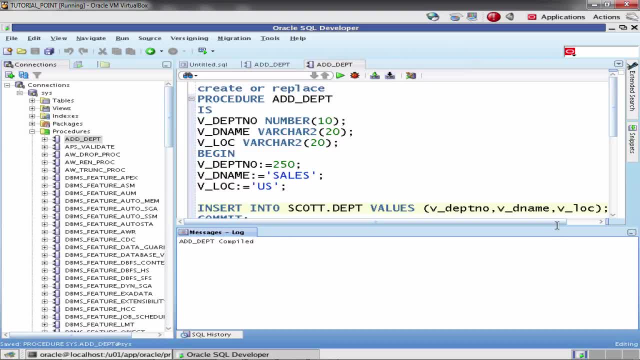 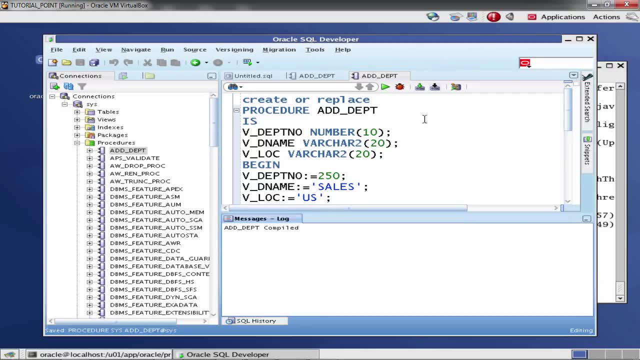 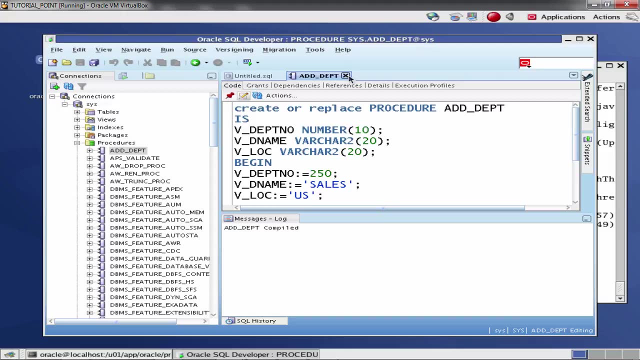 So just compile. fine, So this compilation is completed now. so no syntax errors are there. so now next, what you need to do is, Once the procedure is created and compiled successfully, next is execution of the procedure. fine, So how to execute this procedure? 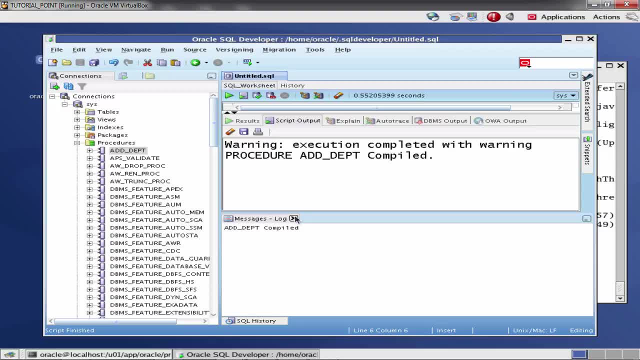 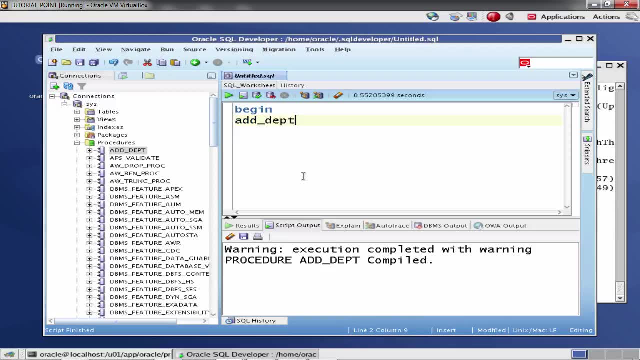 So if you want to execute the procedure simply, you can just write down the code: begin, add dept bracket and end, fine, And here You can just initiate. Ok. So essentially write down, set server output on, fine, and here just execute this procedure. 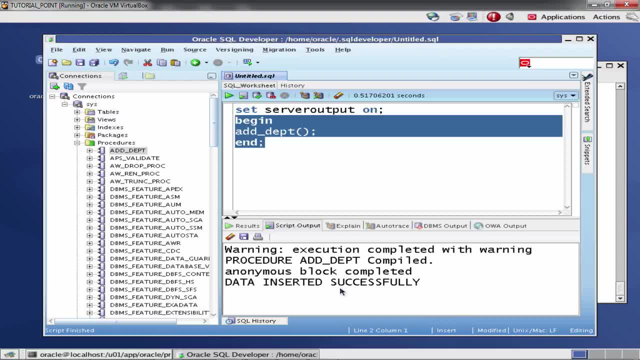 data inserted successfully, you can see. So if you want to just see the output for the dbms underscore output dot put line, you need to just write down set server output on. So that is going to be Display the output of your dbms underscore output. fine, 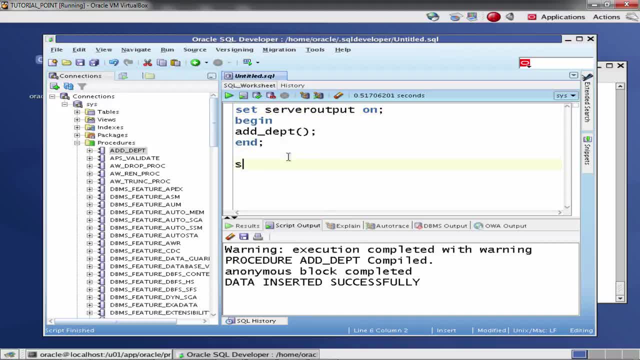 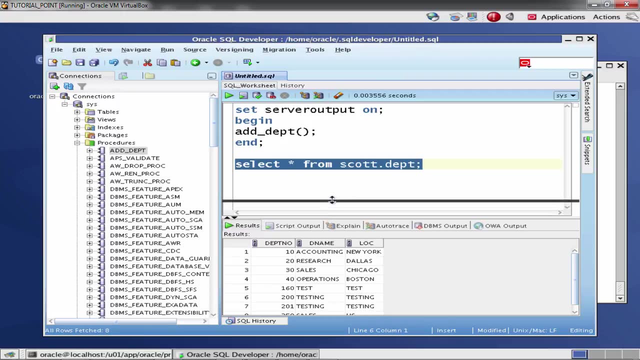 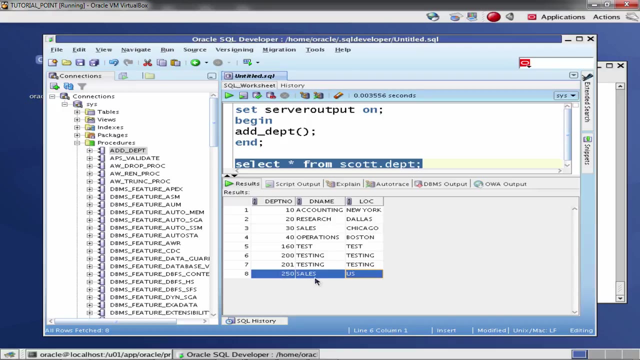 So data inserted successfully. So let's check whether the data is inserted successfully or not. so let's start from score dot dept. so here you can just execute the statement and here you can see says fine. So In this way we can just insert the record using procedure fine. 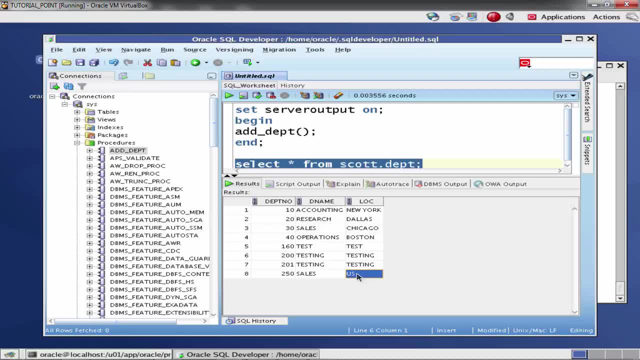 So the important thing is that whenever we are comparing this procedure with the anonymous block procedure, once you are just creating, after that you no need to compile it again, you need to just execute it again. If you are doing any kind of changes, then and then. 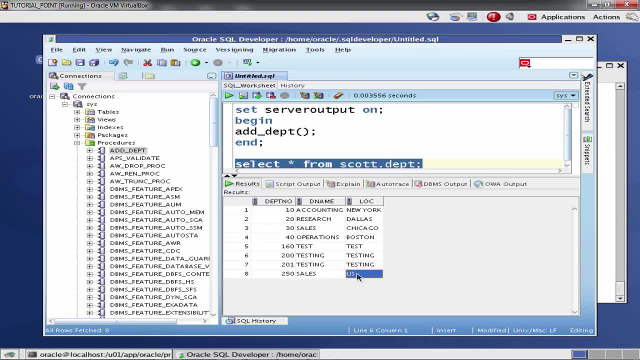 You require to be compiled, otherwise compilation is not required. you need to just execute, and whatever the task is- you know just mentioned in the procedure that is going to be executed- and complete your task, fine. The next one is a function. 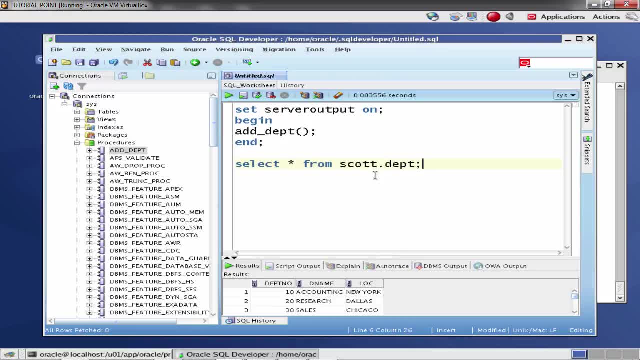 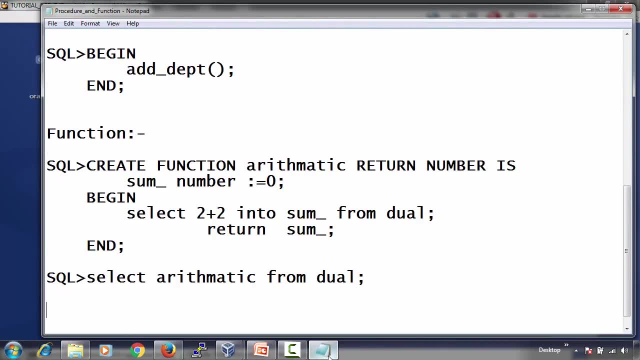 So let's see the function, how to create function and how to execute the function. So function is always written, the value fine. So here we can see, like we are just performing one arithmetic operation, What is the two plus two. So that thing we are just doing using the function. 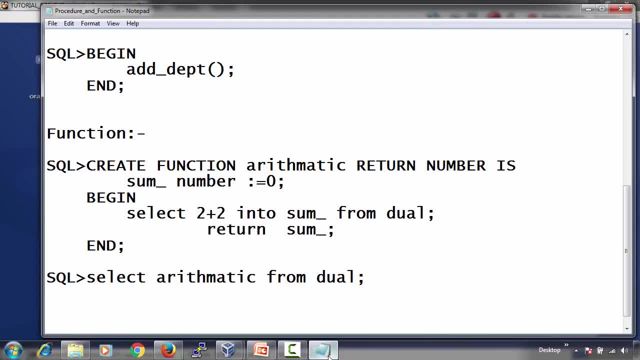 So function is always written the value once, whatever the task you have given to the function, that task is done by the function and it is returning the value. But remember one thing: function is always returning one value, where we are, whenever we are comparing with the procedure. procedure can return the value or cannot be written. 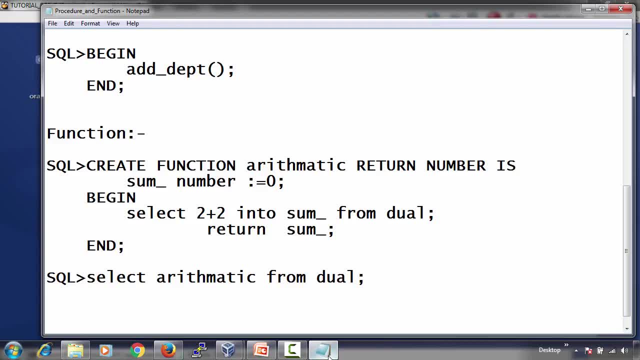 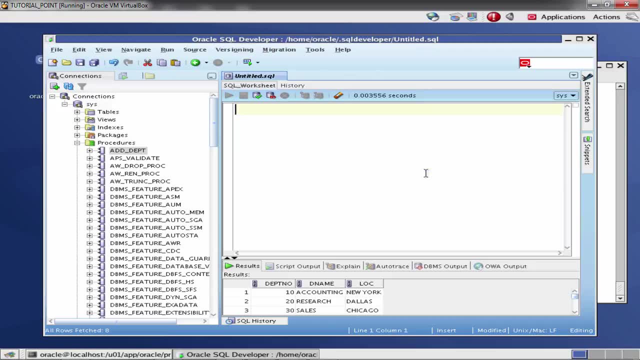 the value. that depends upon the parameter you have given, the output parameter you have given. So let's see how to create function. So here Create or replace function, and here, once you have given this- I am just initially the first time is that? so I am just giving the create function, fine, 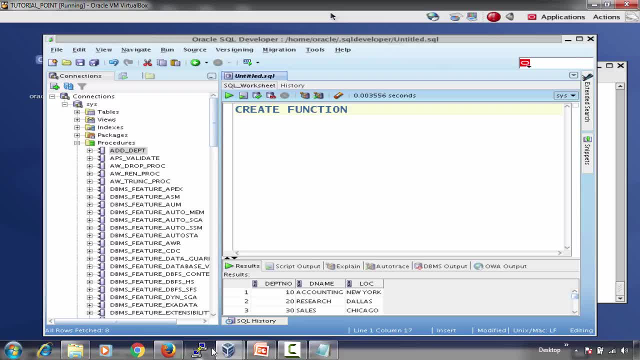 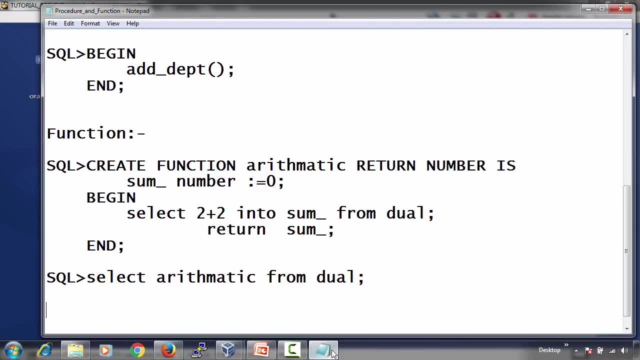 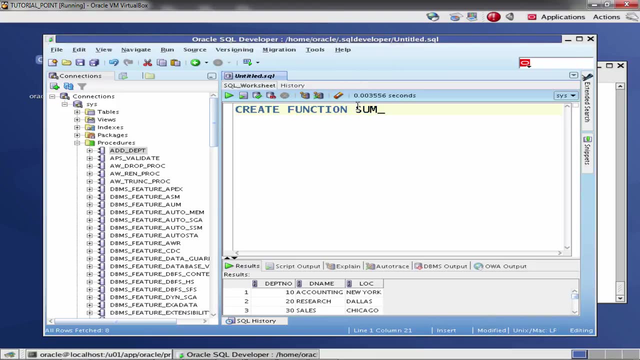 So, and after that I am just giving the name of the function: Arithmetic. So basically it is doing the arithmetic operation or some whatever the you are performing, like some you are doing. So just give the sum, Fine. So here I am just giving the name, some underscore, fine. 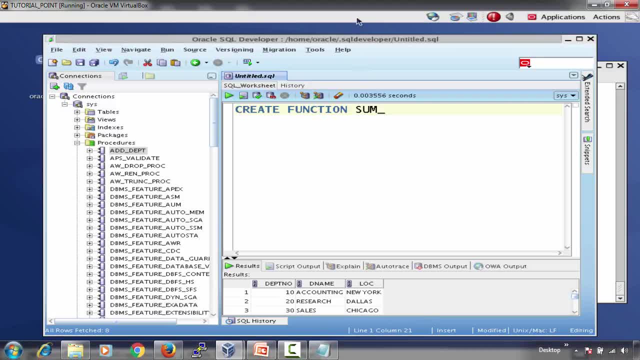 And next is wanting to do some underscore, and the next is return number. is because it is returning the number, So it is just write down the data type, whatever the return, whatever the you are returning: return number, Fine Sum, underscore number equal to zero. 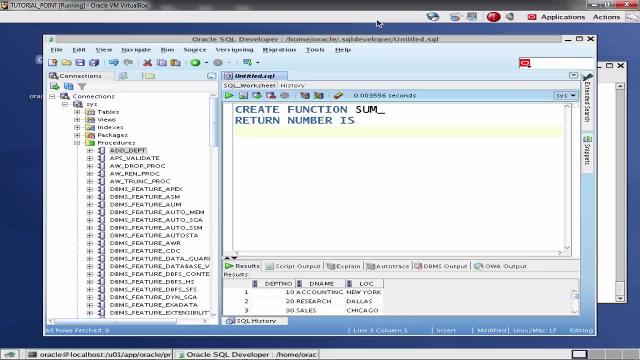 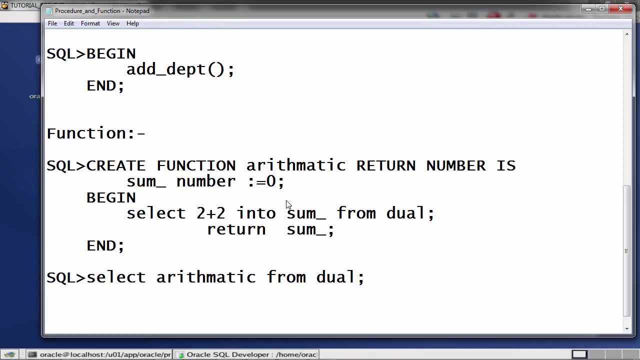 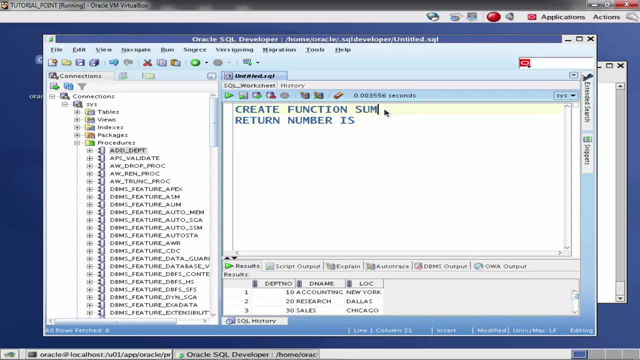 So initially you are just giving the number. So let me just change the name because it is creating the confusion. So arithmetic and sum underscore. So it is creating the confusion. So Arithmetic And Number Number Equal to zero By default.